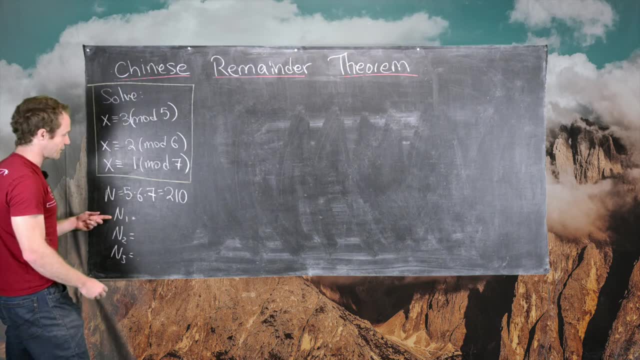 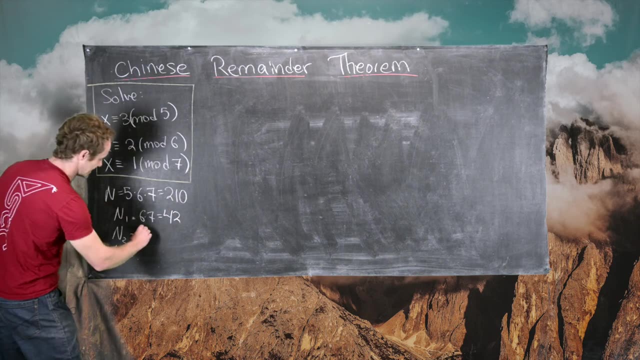 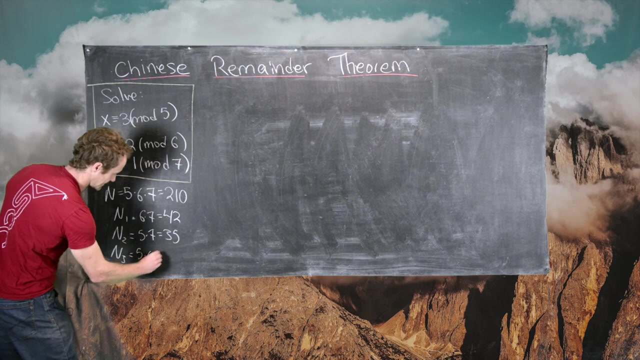 first two, so we're leaving out the third. So here we have: N1 is 6 times 7,, so that's 42,. N2 is 5 times 7,, so that's 35, and N3 is 5 times 6,, so that's 30.. So now we're all set. We have 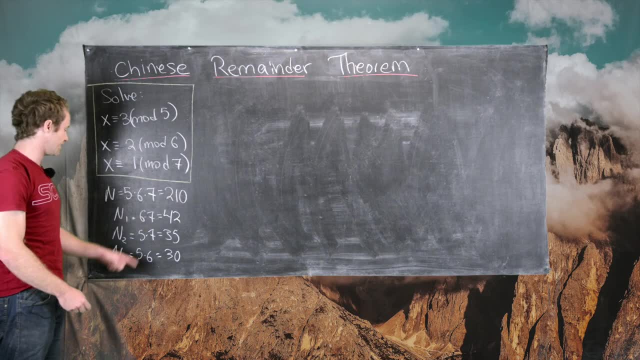 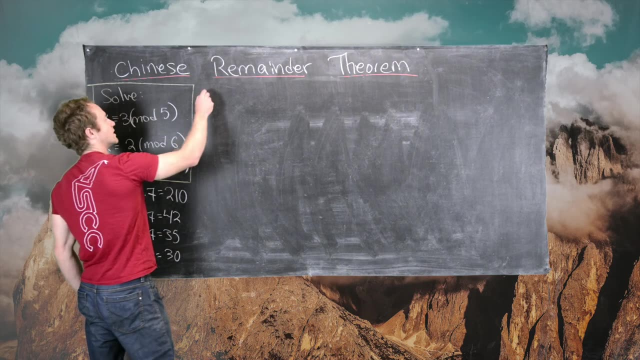 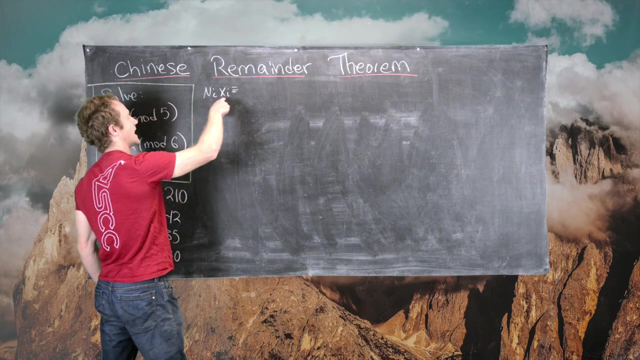 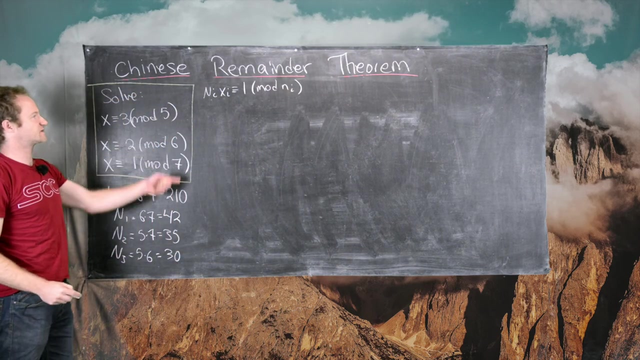 these numbers to work with. So the next thing we want to do is invert n i modulo little n i. So in other words, we want to solve the linear congruence. capital N i xi is congruent to 1 mod little n i, where the capital Ns are given here and the small 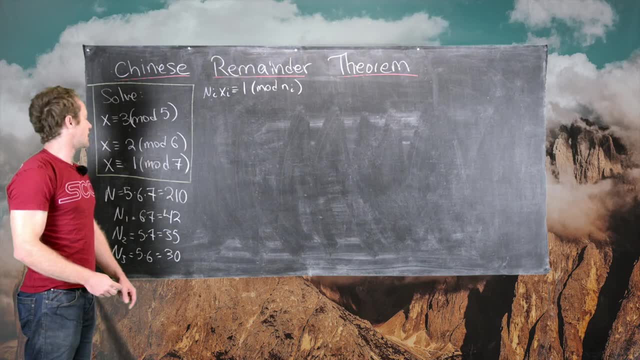 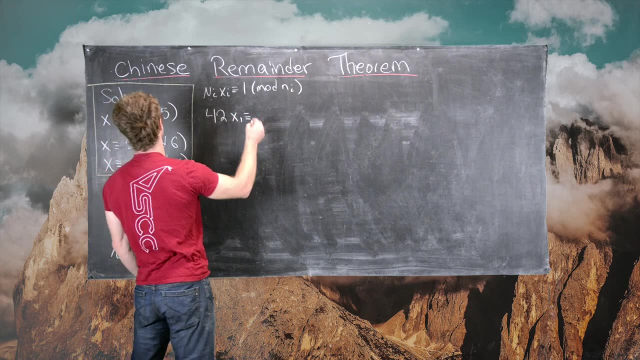 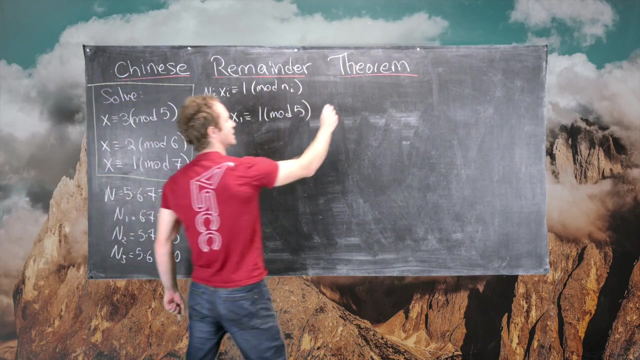 Ns are given here. So that means we have three things to invert. So we need to do. 42 x1 is congruent to 1 mod 5.. Good, We need to do. 35 x2 is congruent to 1 mod 5.. Good, We need to do. 35 x2 is congruent to 1 mod 5.. Good, We need to do. 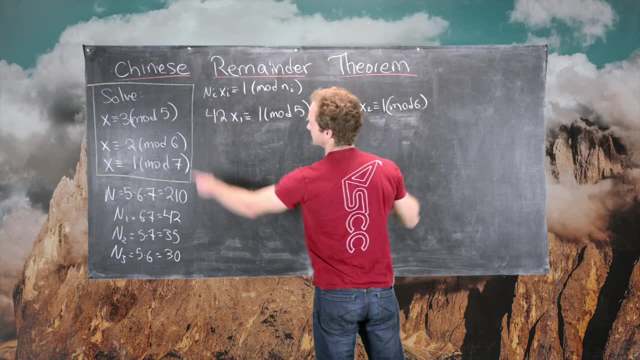 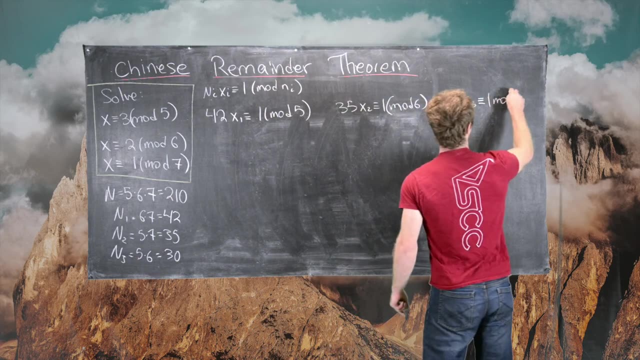 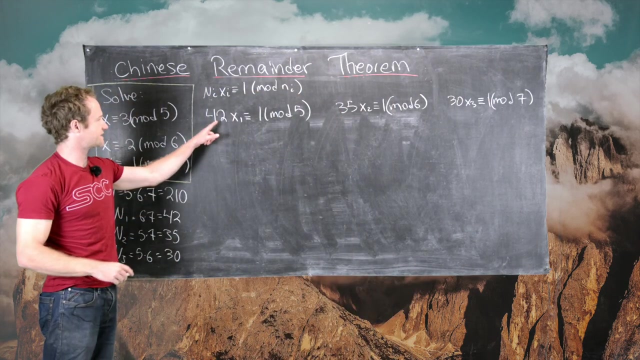 45 x3 is congruent to 1 mod 6.. So that would be the second. And finally we need to do: 30 x3 is congruent to 1 mod 7.. Okay, so, before doing these calculations, it's probably best to simplify these. 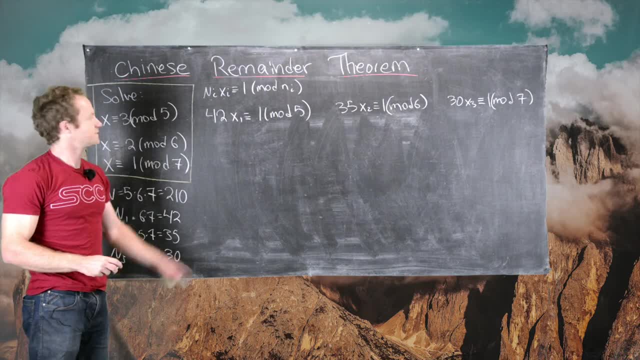 numbers modulo 5,, 6, and 7 as appropriate. So here we have: 42 is the same thing as 2 mod 5, so we can write 42 x1 as 2 mod 5.. So we can write 42 x2 as 2 mod 5,. so we can write 42 x1 as 2 mod 5, so we can write: 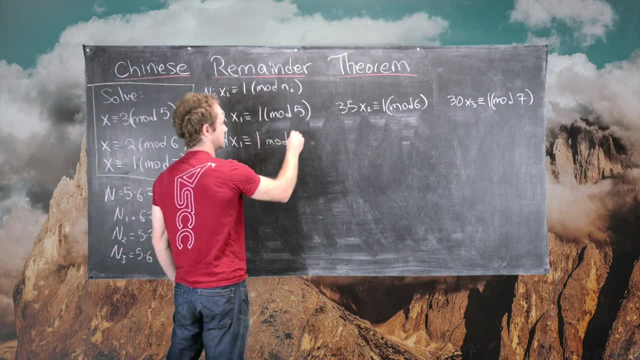 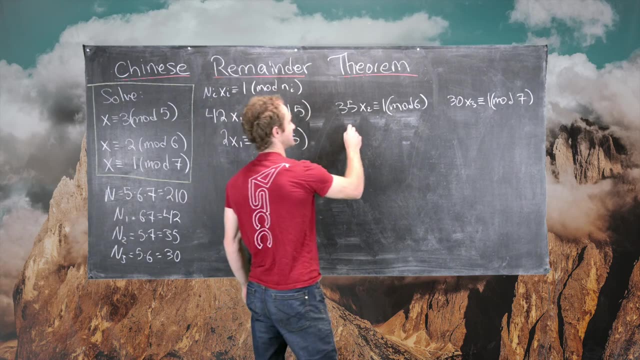 42 x1 as 2 mod 5, so we can write 42 x2 as 2 mod 5,. so we can write 42 x2 as 2 mod 5, so we can write 42 x1 as 2 x1 mod 5, and then so on and so forth. So 35 is the same thing as 5, so here we have 5, x2 is 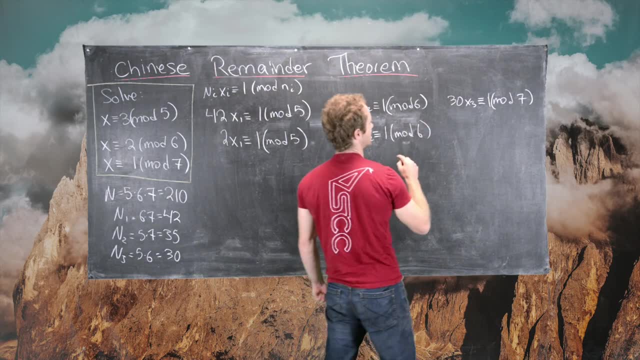 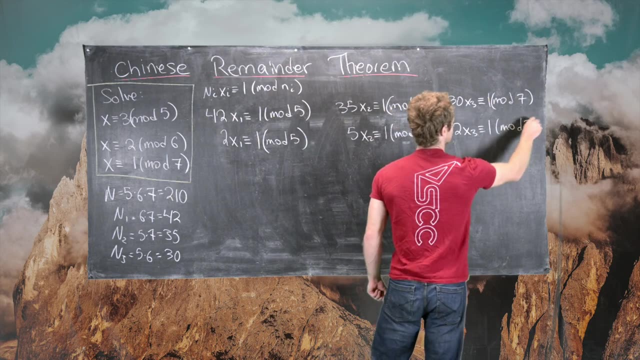 congruent to 1 mod 6, and here we have 30 x3 is the same thing as 2 x3 mod 7.. And now, since 5,, 6, and 7 are pretty small, we can guess and check until we have inverse. 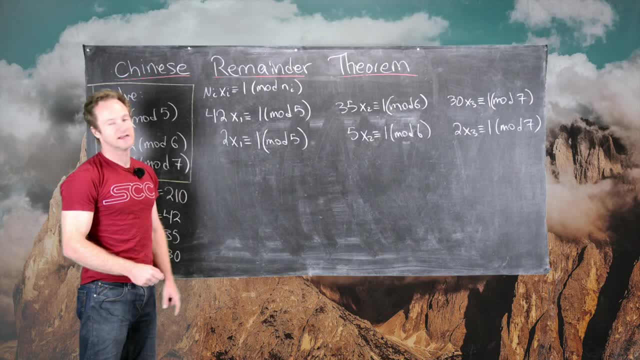 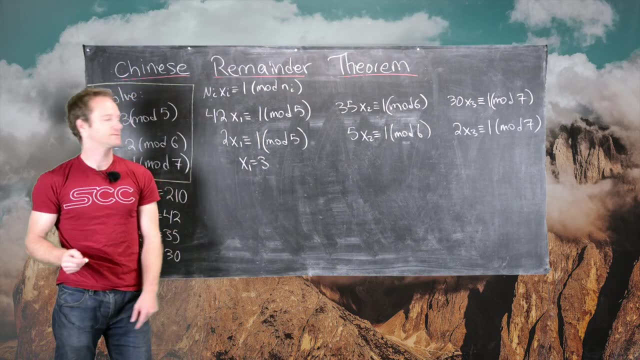 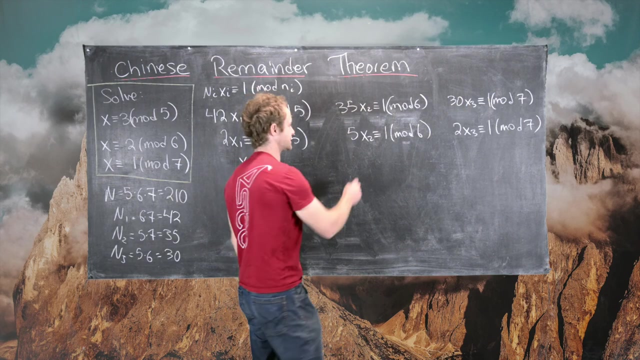 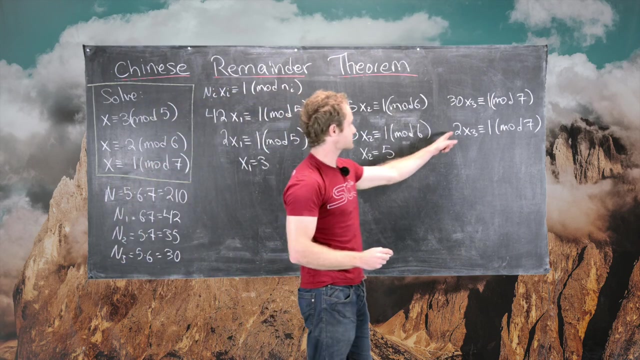 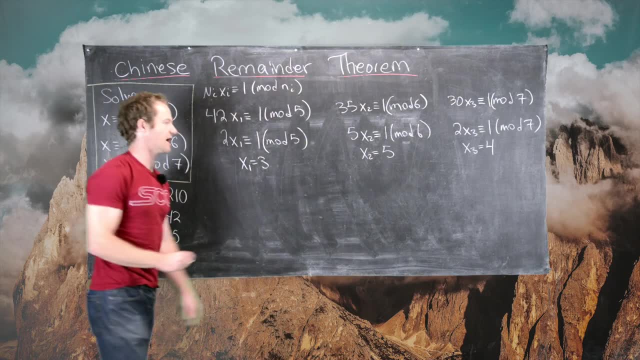 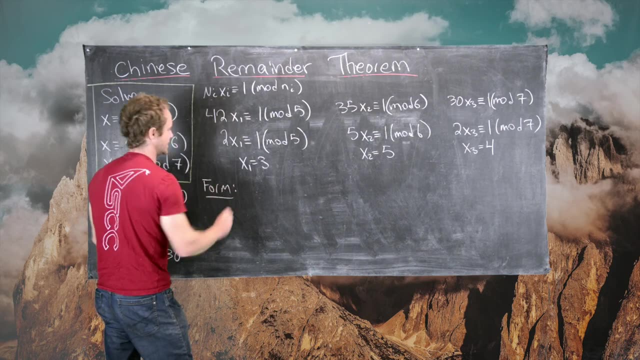 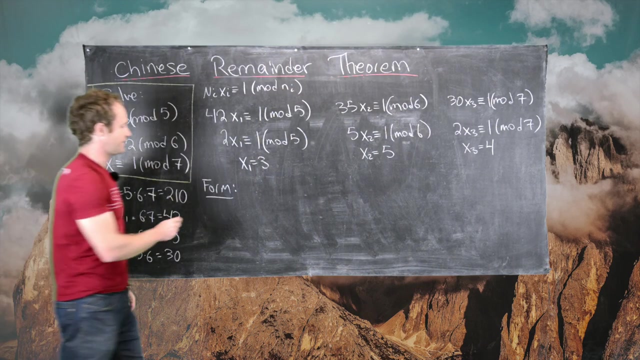 equal to 4.. Good, So now we have x1,, x2, and x3. And then now we form the following combination of the xi's, the capital ni's and the bi's which are in this column. So we want to form x. 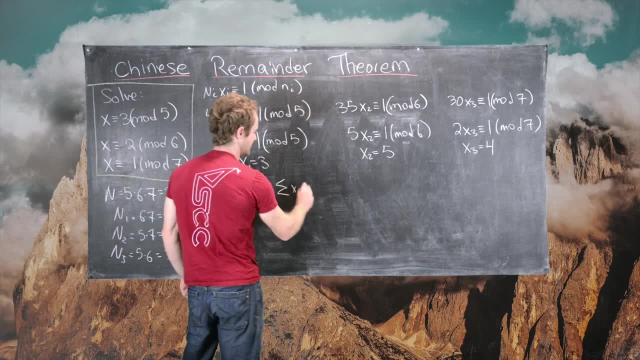 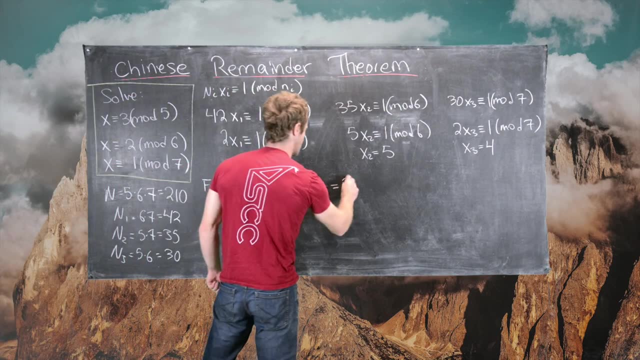 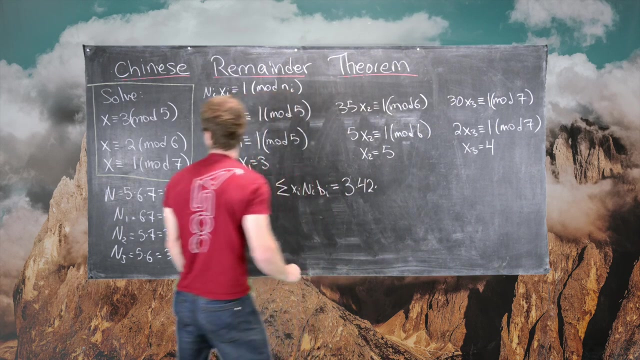 which is the sum of the xi, the ni times the bi Good. So let's see what we get there. So we'll start with 3, so that's x1 times n1,, which is 42, times b1,, which is 3,. 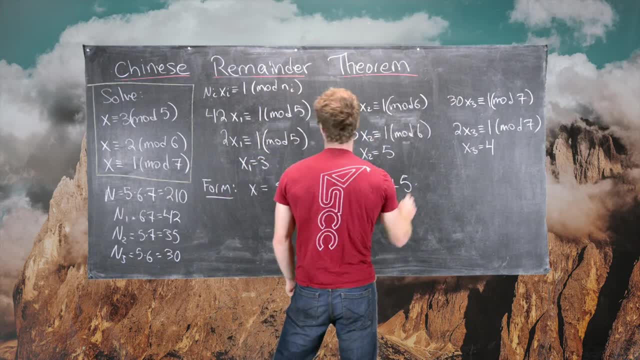 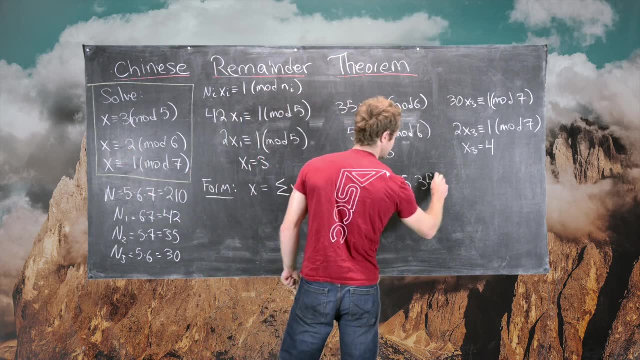 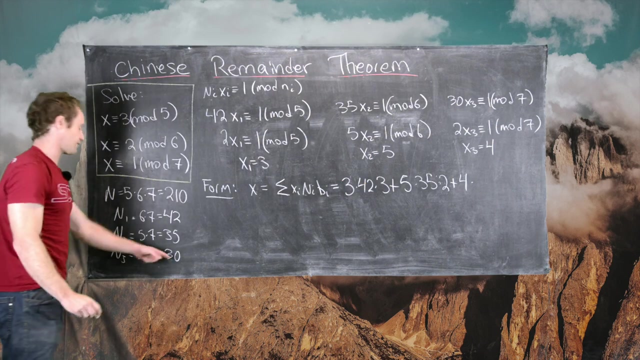 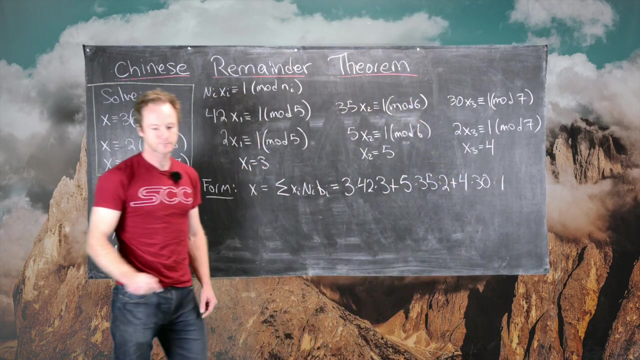 plus x2, which is 5, times n2,, which is 35, times b2,, which is 2, and then plus x3,, which is 4, times n3, which is 30, times b3,, which is 1.. Okay, Good. So now that we've got this number calculated, 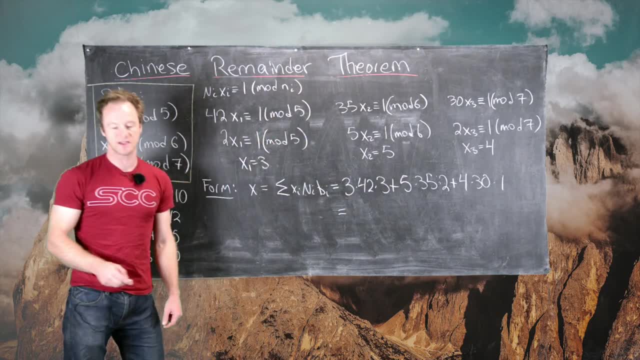 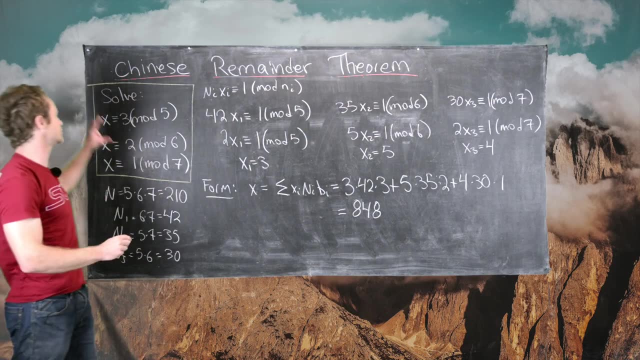 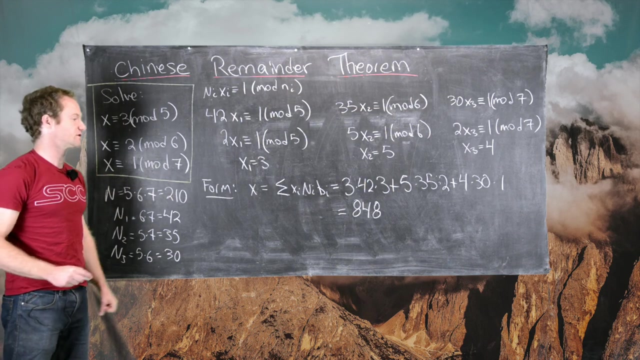 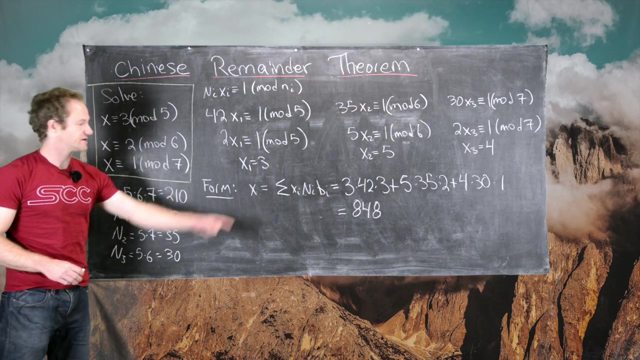 we can do the arithmetic and we notice that this is equal to 848.. 848.. So 848 is a solution to this system of linear congruences. but we know that this solution should be unique modulo capital N, so modulo 210.. So that means we'll reduce 848 modulo 210,. 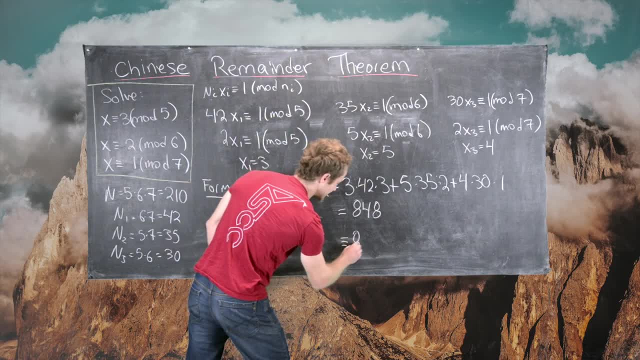 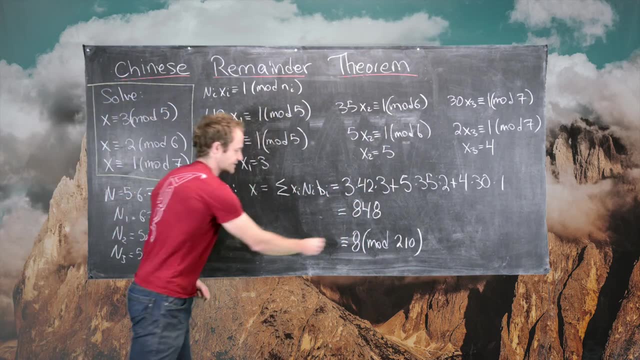 and we'll notice that this is congruent to 8 mod 210.. And that's our final answer. So we have x is congruent to 8 mod 210..